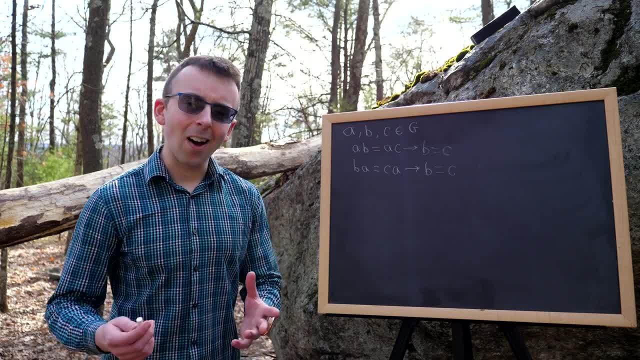 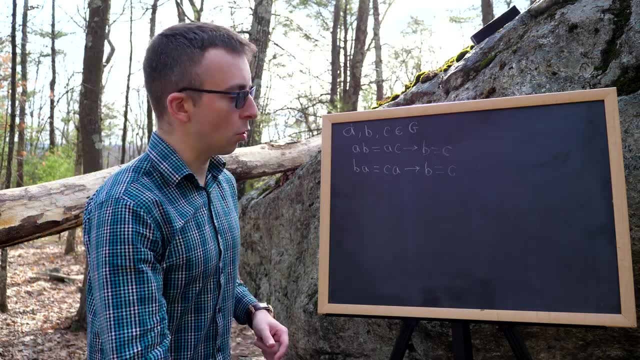 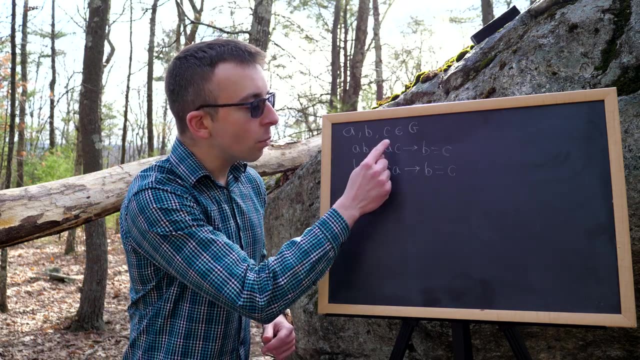 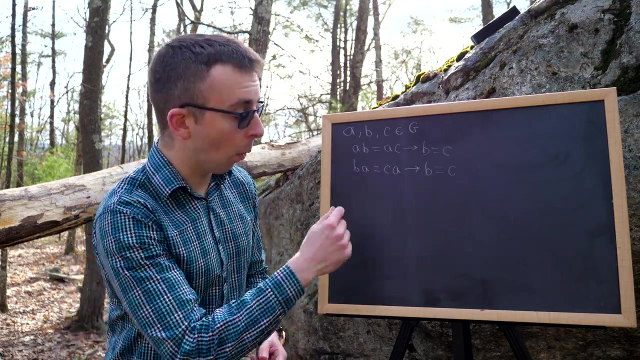 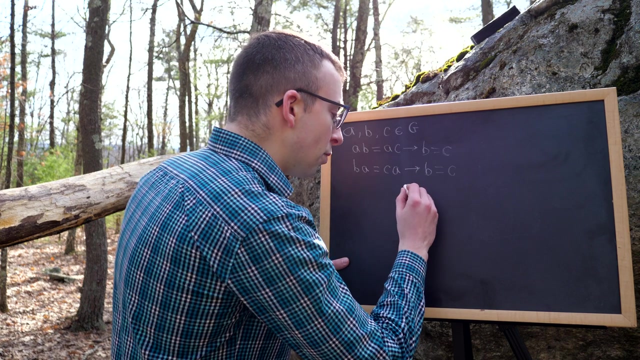 have to do. So today, we're going to prove something that we've been using all our lives, a very familiar result, which is the cancellation law, which tells us this. It's a result about groups. If we have three elements, A, B, and C, from a group G, and we know that A, B equals A, C, or we know that B, A equals C, A, we can cancel the A's on the left or cancel the A's on the right to conclude that B is equal to C. This is something you've used a lot, of course. 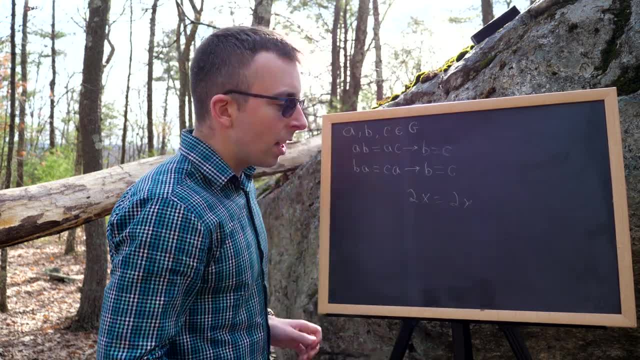 If I tell you that 2X equals 2Y, you would probably not hesitate to cancel out the 2's and conclude that B is equal to C. 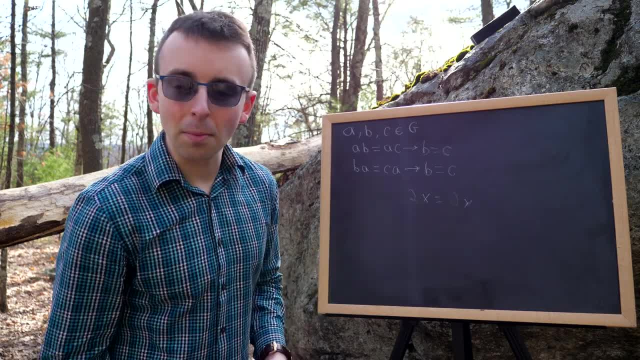 You would probably not hesitate to conclude that X is equal to Y. My finger doesn't make a very good eraser, but you see what I mean. You would be perfectly content to do that. The thing is, 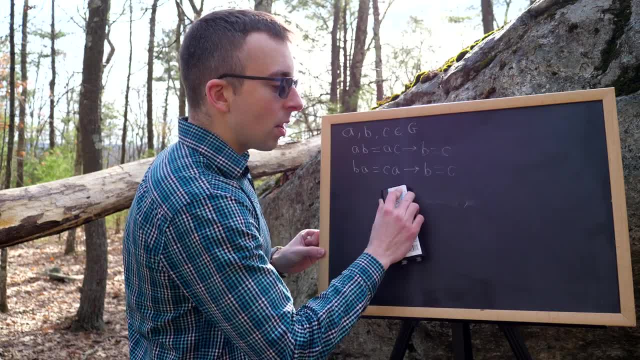 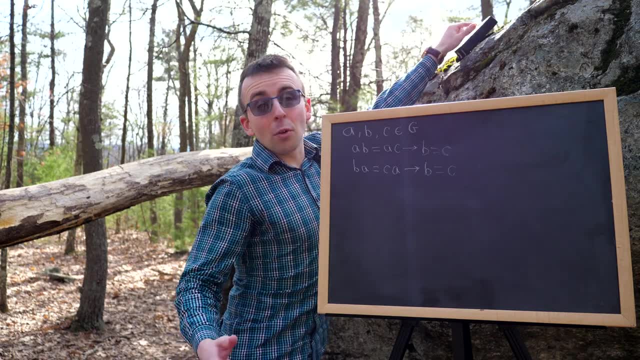 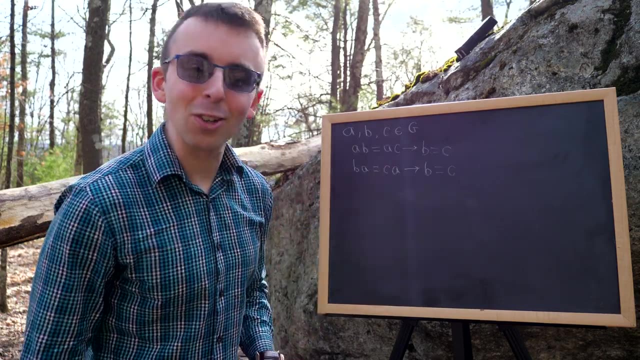 when we're studying abstract algebra, a lot of times we are considering arbitrary operations on arbitrary sets. So we don't necessarily know that everything works exactly the way that we would like it to. So let's go ahead and prove this so that we can use the cancellation law going forward for group elements. 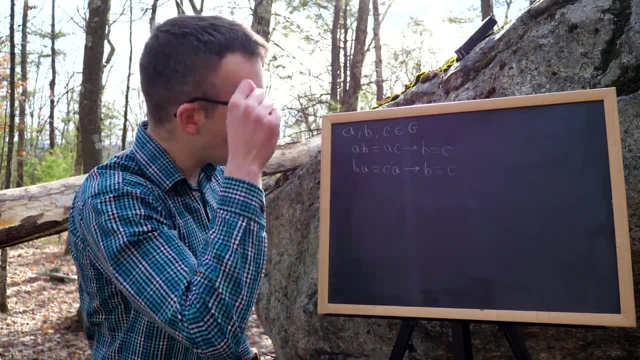 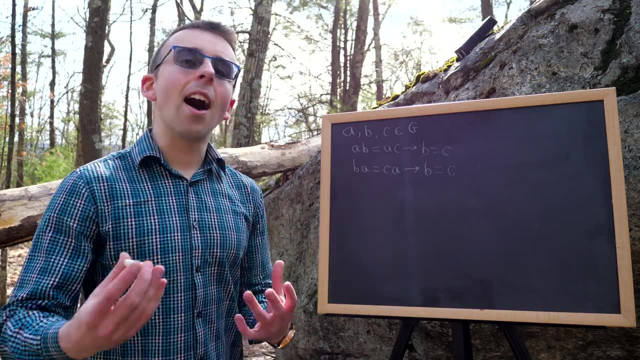 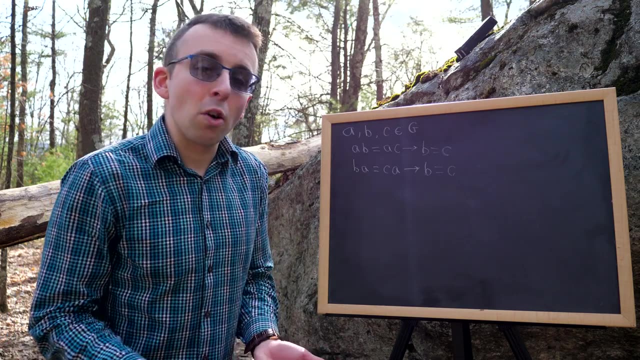 If we've got the same element being composed on the left, we can cancel it. Or if we've got the same element being composed on the right, on both sides of an equation, we can cancel it. Now, I'm going to say times to indicate this operation. I'm going to talk about it as if it is multiplication. Just remember, it's an arbitrary operation, but the words we use to describe multiplication are nice words. So I'm going to keep using them. 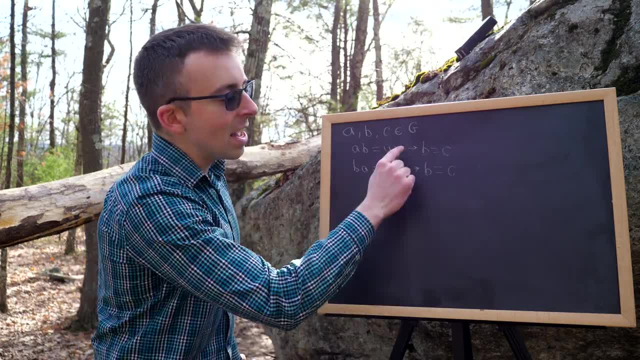 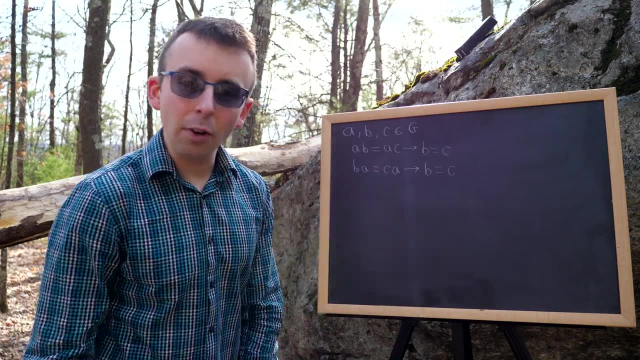 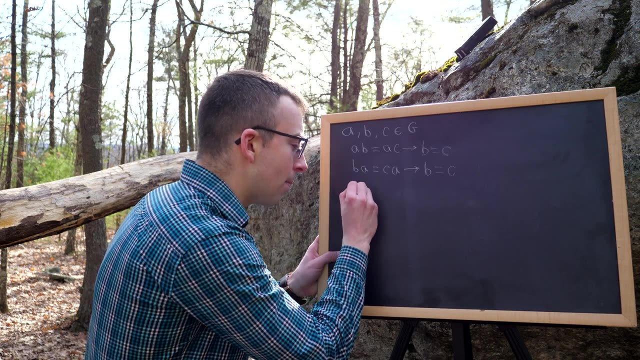 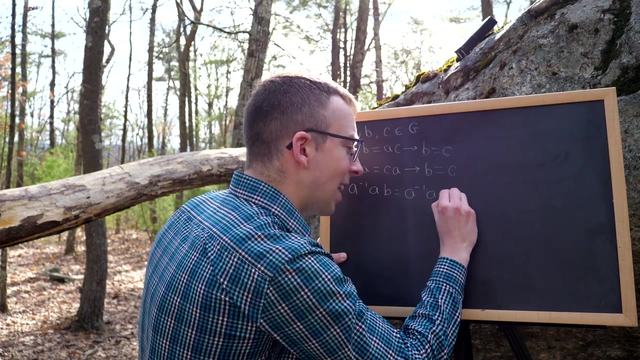 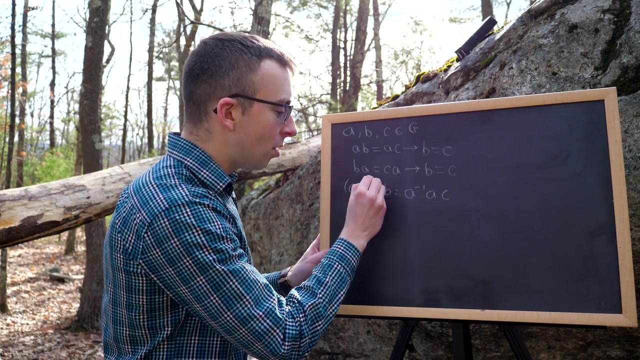 First, let's prove this one, that A, B equals A, C implies that B equals C. It's super straightforward. Since this is a group, we know that A has an inverse element. So we can multiply both sides of the equation by A inverse on the left. If we do that, we get that A inverse times A, B is equal to A inverse times A, C. Now we can use the perhaps underappreciated group property of associativity to associate the A inverses with the A's. That way, we can convert them into A's. So we can get the A inverse times A, B's. So we can get the A inverse 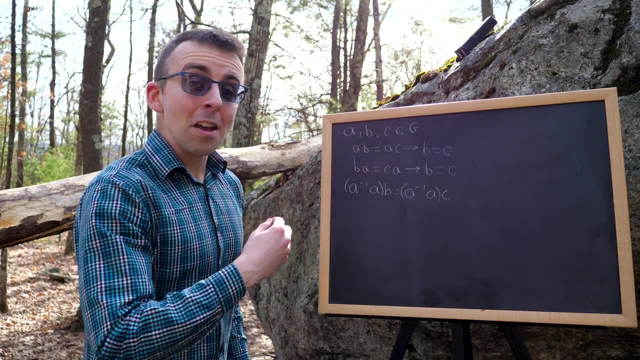 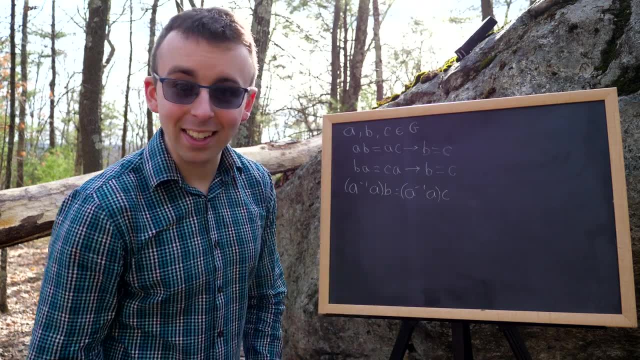 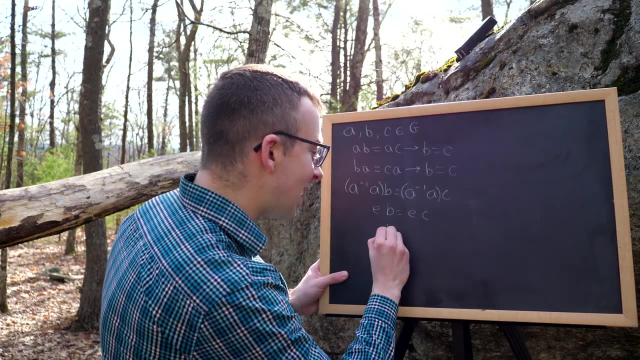 times A, B's. So we can combine those before we worry about anything else. By definition of inverse elements, of course, this is going to be the identity, which we'll call E, and this will be the identity, which we'll call E. Thus, we have that E, B equals E, C. And then by definition of identity element, we conclude that B is equal to C. So indeed, we can cancel 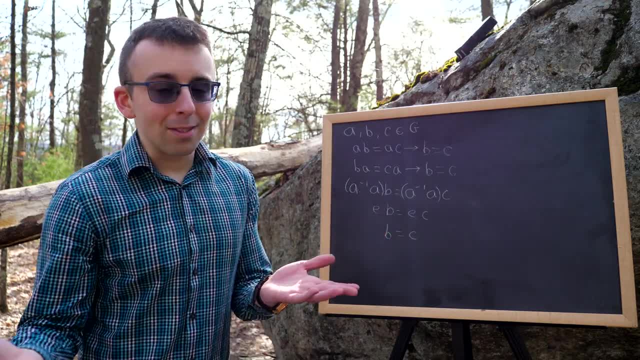 elements on the left. Now let's prove this one. Of course, it's basically the same exact proof that if we've got B, A, 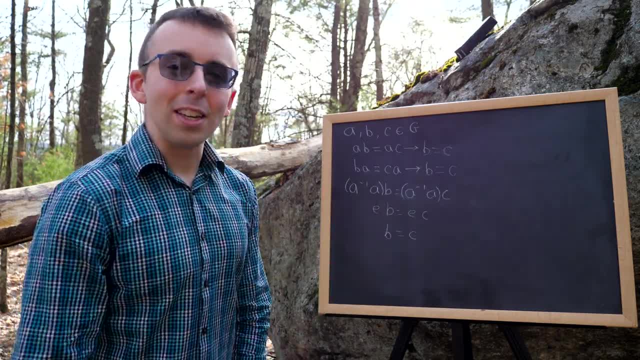 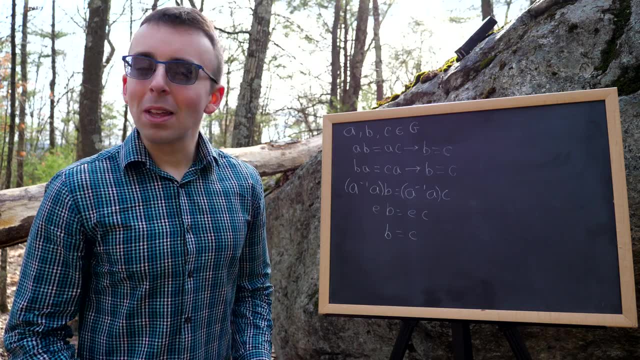 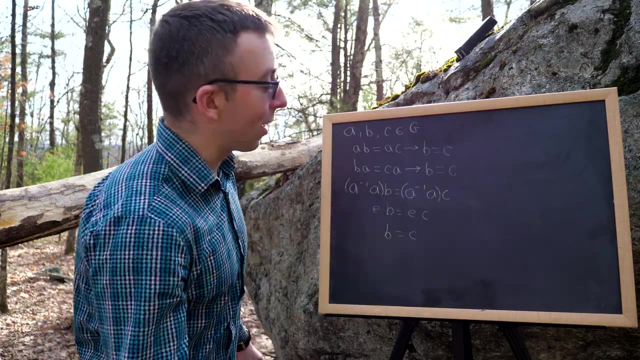 equals C, A, we can conclude B equals C. We're going to do the same magic trick. We'll just multiply on the right by A inverse. Man, it sounds like I chose to film next to a war zone or something, but I promise you I didn't. At least I hope I didn't. So again, we know we got inverse 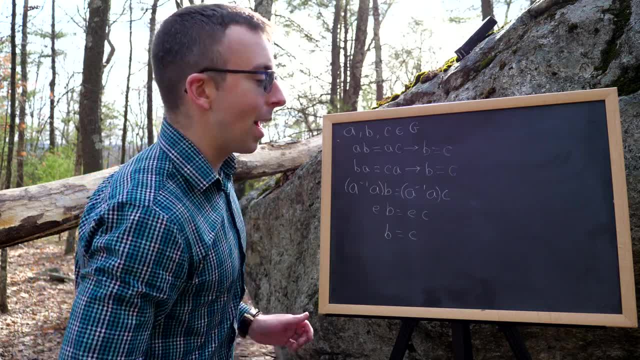 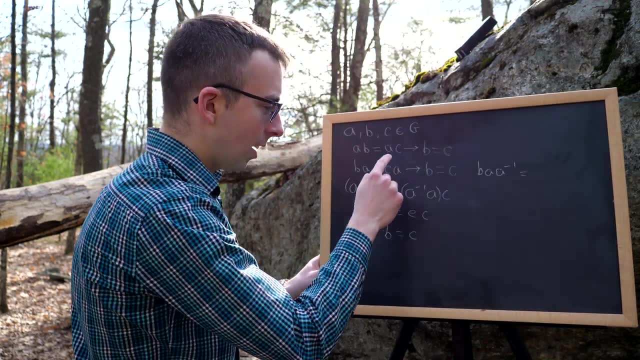 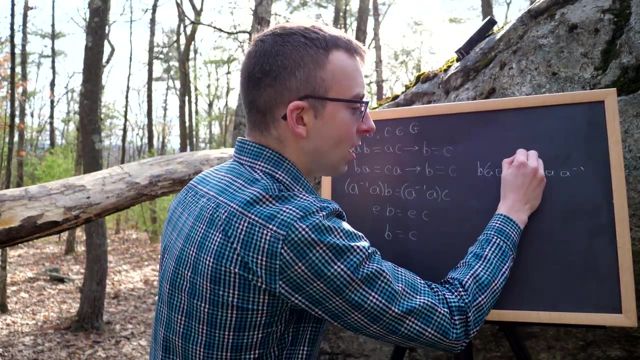 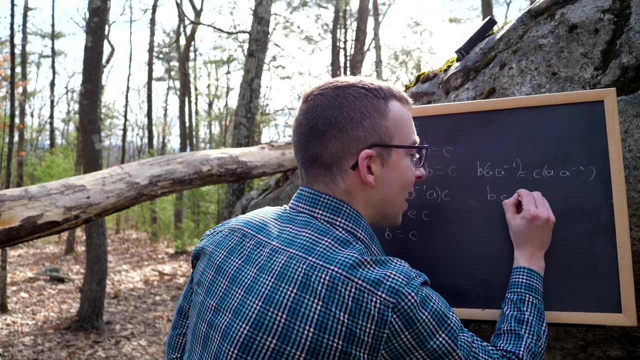 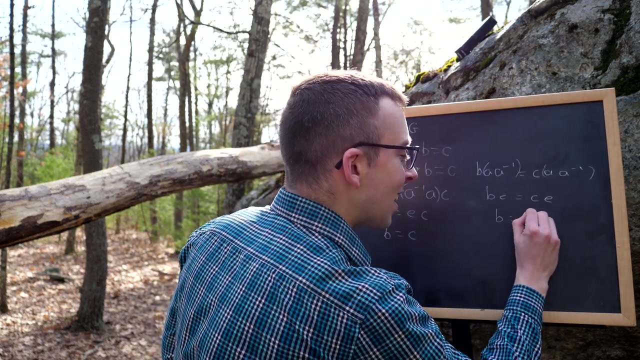 elements. So we'll multiply both sides of the equation on the right by A inverse. That's this equation here. Now, if we do that, we get that B, A, A inverse equals C, A, A inverse. C, A, A inverse. Again, we can use associativity to associate A with A inverse. Those will produce the identity elements. And so we have that B times E, the identity, is equal to C times E, the identity. And then by definition of identity, we again have that B is equal to C. 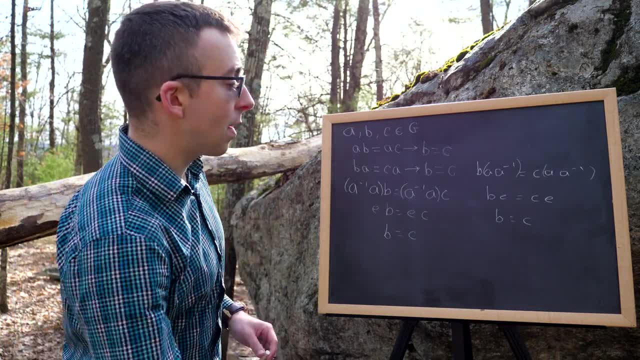 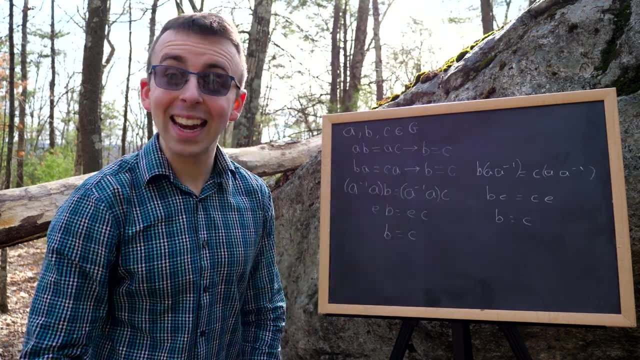 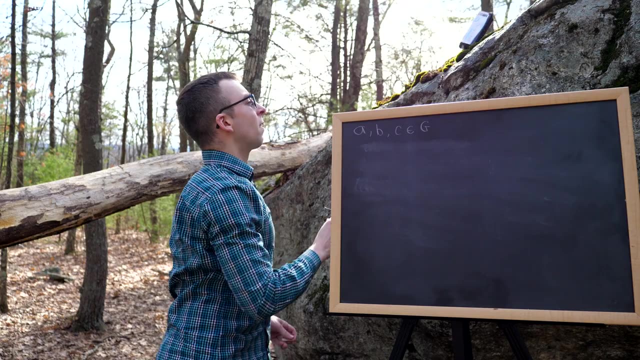 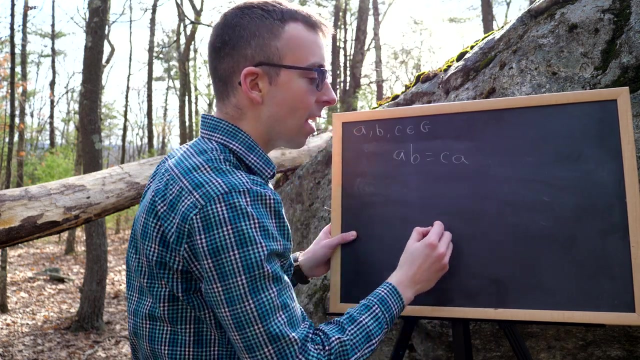 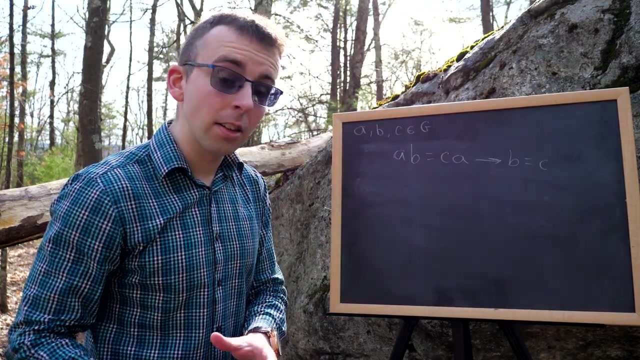 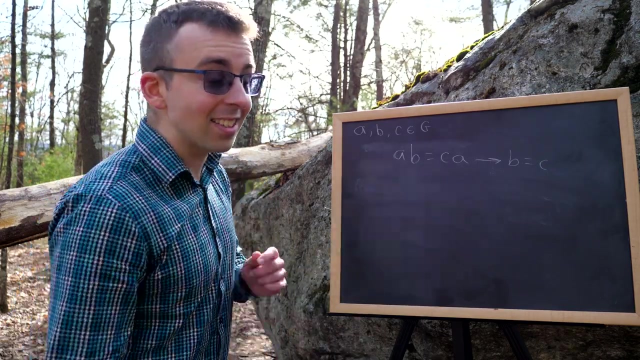 So now we know we can use the cancellation law for groups. If we have the same group element composed on the same side, on both sides of an equation, either on the left, or on the right, we can cancel it out. One thing that you should notice is something that we didn't prove here. What didn't we prove? We didn't prove that if A times B equals C times A, that we could then conclude that B equals C. A has to be on the same side on both sides of the equation. Either it has to be on the left on both sides, or it has to be on the right on both sides.